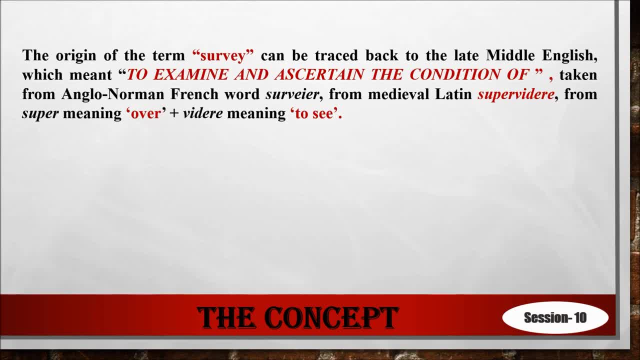 looking here again is the same idea of a field survey. that is about going to the ground and seeing it self. like we go to the ground physically and look for the details to ascertain, to examine the conditions of the ground ourselves. so that is the basic idea behind the term survey itself. 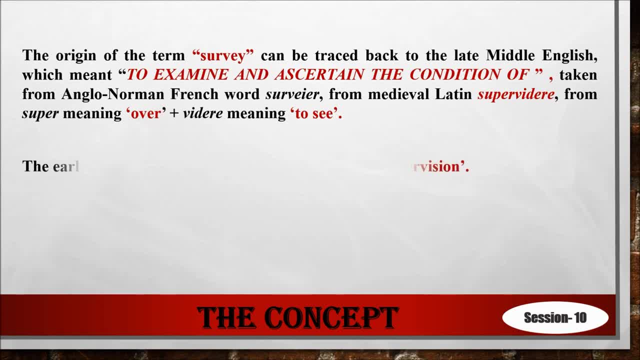 so the earliest sense was basically supervision. around 15th century, in common era, the idea was to supervise what is happening on the ground. that is what is the basic meaning of a survey that still happens. the survey of india that does census of india that does census and server of india that. 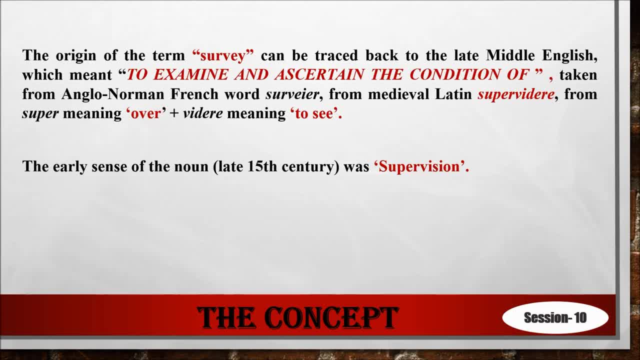 does different kinds of surveys right. that prepares our topographic sheets. so they do what. they supervise. what is going on the ground? what are the changes happening on the ground? isn't it in terms of population or any physical structure or the infrastructure? isn't it so? all these features? 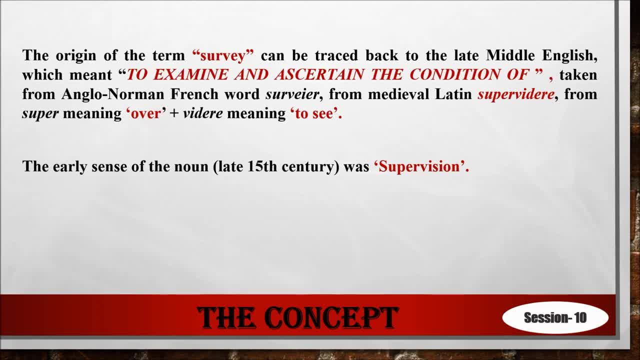 what is happening on the ground, what they basically supervise, these agencies? so when we go to the field for our survey, we do the same work, taking our objectives into mind. we go to the field and supervise first ourselves to ascertain and examine what exactly is the ground condition. 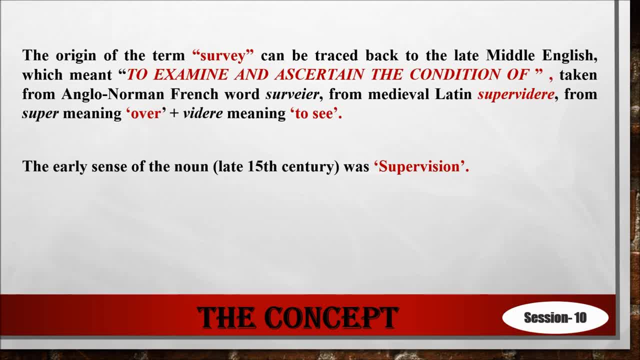 related to our objective of the work. so it has been widely used in geographical research as a test and it is a very systematic technique of investigation and this is through direct observation of the event, the phenomena right, and it is very systematic gathering of data that we must remember. it's not randomly gathering any information, but the information that we gather. 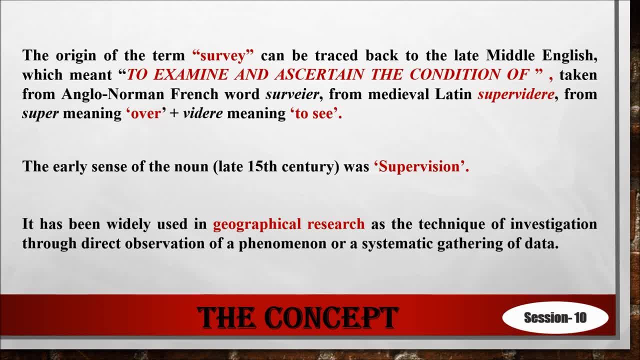 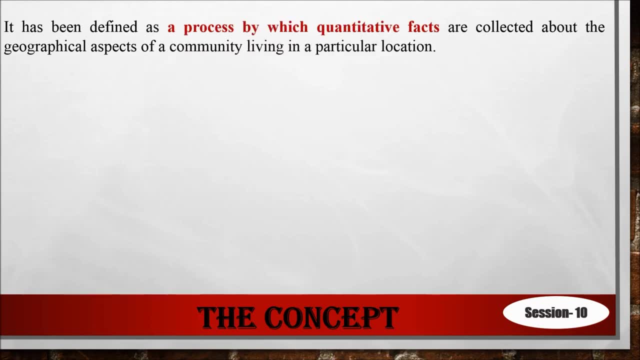 has a system involved. it means it has a basic flow involved in which we can gather different data sets from the field work. so this is about the basic concept. then further, if we see it has been indicated in the field, we can see that the way is the fact that the self-draft data is collected. 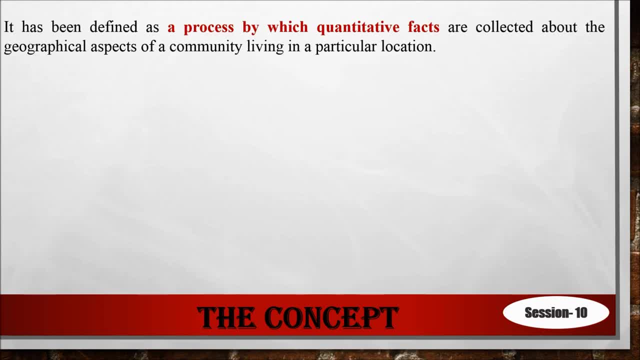 by these data sets and by using these data sets, we can understand how these data sets are collected, but there are factors by which quantitative facts. now you understand that the facts are quantitative in nature. when we collect geographical aspects, asking from a community their responses, isn't it? so we try and quantify those factual informations in the field. that's how it has been. 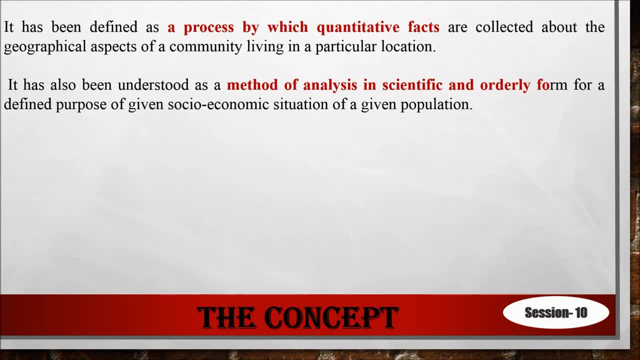 defined basically, but if we can also understand that basic definition about it, so it has also been understood as method of analysis in scientific and orderly form. so scientific nature. remember we have already talked in the previous sessions that it has the rational of being scientific and orderly. so it is important in order to give 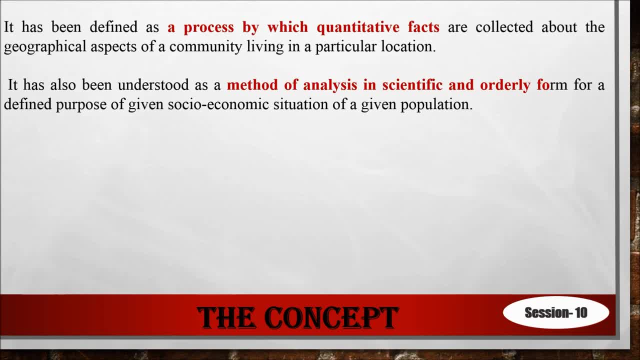 purpose to what we are studying, for example, socio-economic condition of a given population in the ground. right then, field survey is an important tool to gather evidences related to certain socio-economic and geographical conditions. problems event, isn't it? so this is what is what we study. so the term socio-economic survey, many times is interchangeably used. 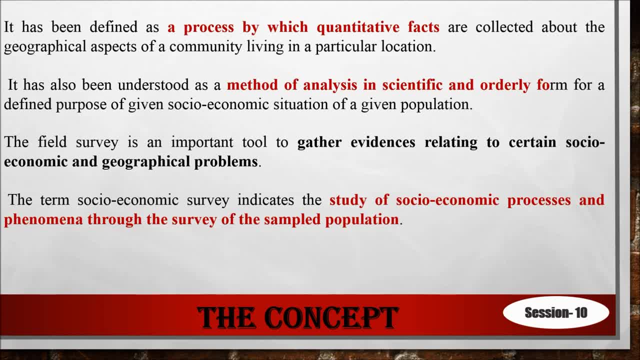 with the field work like, because study of socio-economic processes and the related phenomena. right, geography is all about interrelations, so what we study is the socio-economic conditions, the processes operating and how it is linked with that particular physical location, physical, uh, the place where we are looking at, isn't it so this phenomena with physical factors and 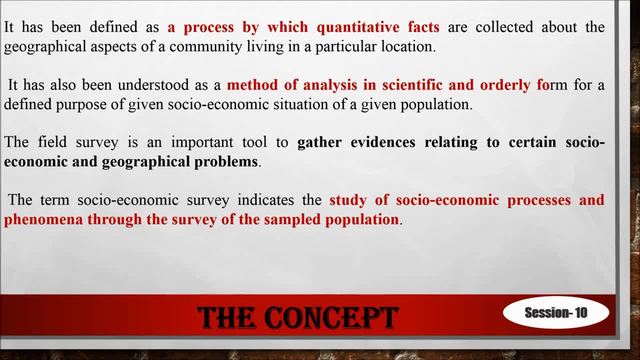 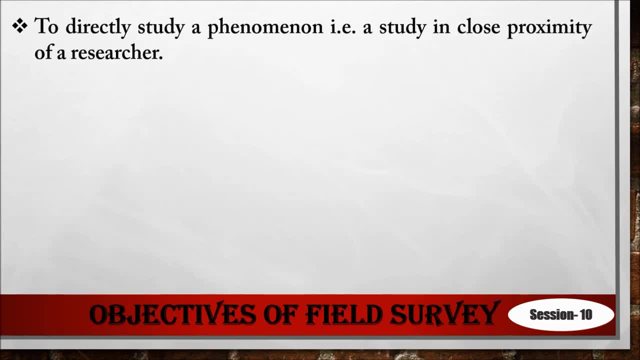 socio-economic factors. that is what we study in the sampled population, in geography, right, so let's understand the objective of field survey. so the objective of field survey is: first objective is to directly study a phenomena. right, empiricism is the basic characteristics, right, so directly we study a phenomena that is in close proximity, in close. 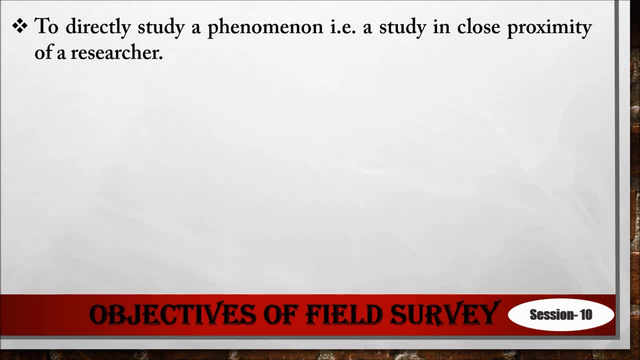 situation with a research scholar. so to collect general geographical information, isn't it? we also collect general geographical information about land, soil, vegetation, agriculture and so many other attributes of geography that we study in physical and as well as human geography is to identify basis for formulation of hypothesis. many times what 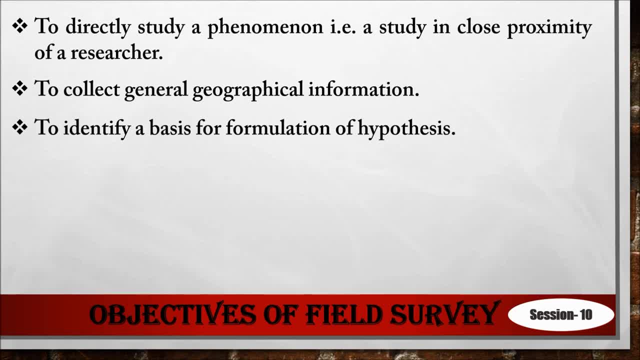 happens, this field work, primary work, also becomes basis for the formulation of a certain hypothesis that we look forward to the broader framework of research. so many research happens that we first make hypothesis based on secondary analysis only. but many a times what happens? that field work gives us our hypothesis formulation. when we go to the ground then we formulate a hypothesis. so 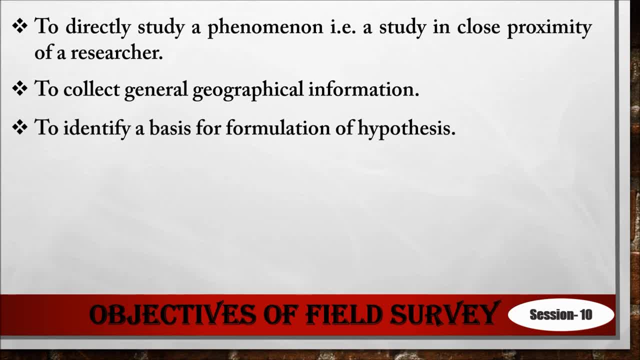 both ways this can be interpreted right. so then, to explain cause and effect relationship. this is one of the basic modes of explanation that we study in geography and ecology: cause and effect. x is the function of y, so very much a functional relationship. what is the cause, so what is the? 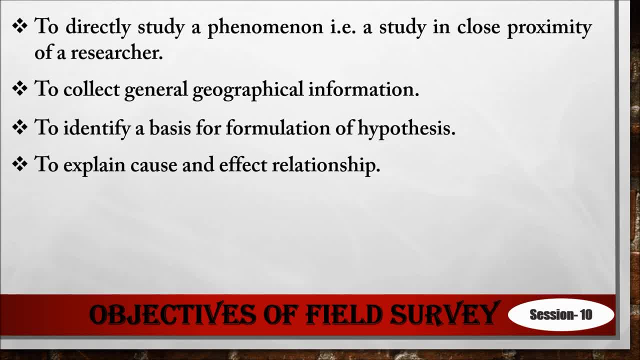 effect, right. so what kind of relationship does the x factor has with y factor? in the field, then, to understand opinion and attitudes of people, that is what we are very much interested in, isn't it? people? because it's always relationship between human beings and environment. so opinion and 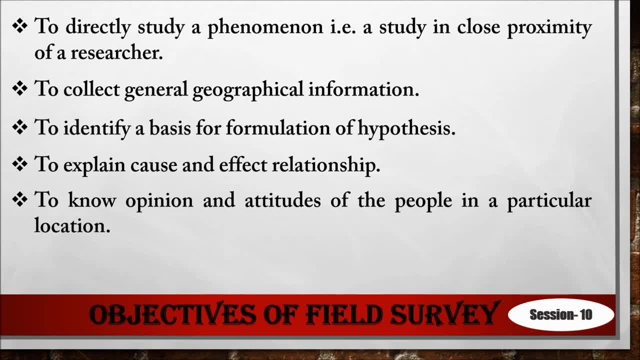 attitudes of people would definitely matter. that's why field work can never go literally leaving the people aside. so somewhere or the other we take into consideration people in our study. that is one of the objectives. some studies may be completely physical. they may not involve people at all. but we are talking about larger objectives of field survey here, not just a physical survey. 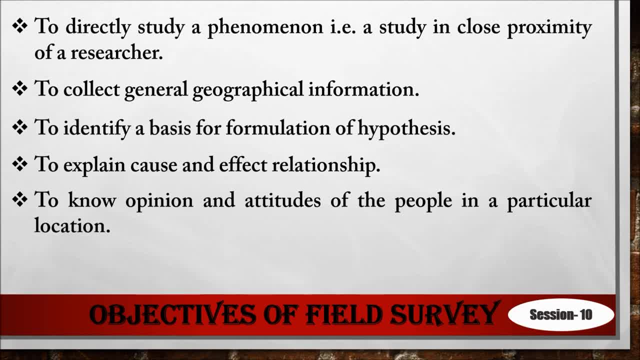 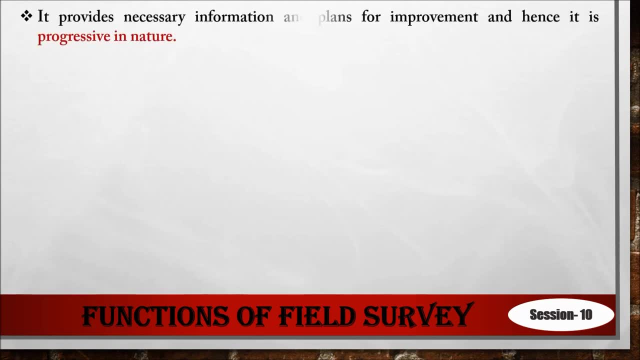 so these can be the maximum output of the entire objectives that we can study together. right? so let's look at the functions of a field survey then. so we already know the objectives of field survey. what are the functions? so basic function is to provide necessary information and plans for. 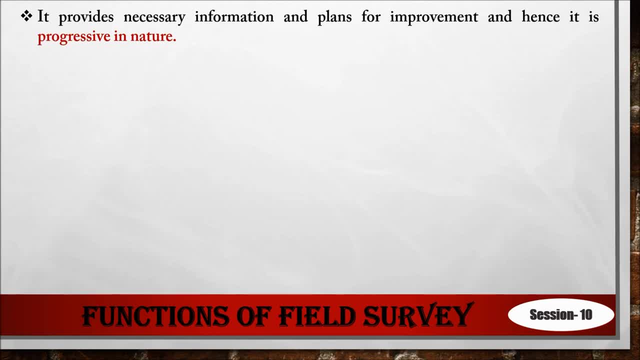 improvement, isn't it? hence, it is progressive in nature. remember, the function of field survey is to be progressive in nature: what is happening on the ground, what are the plans, how we can improve it right, and to collect necessary information about it. so it enables us to interpret, synthesize and 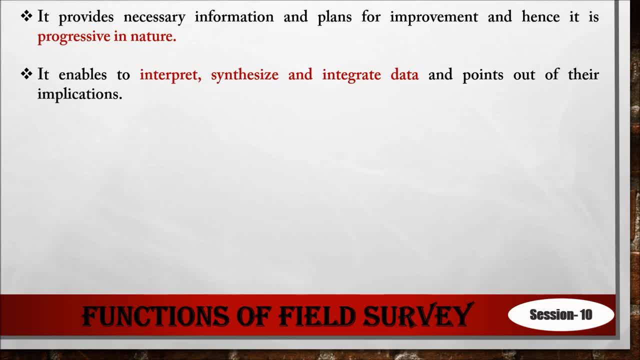 integrate. remember: interpretation, synthesis and integration, these are the three important points for which we set out to the field. so what happens? we interpret it, synthesize and integrate various data and then we come to our conclusion, inferences that we draw from the field. so it is more realistic. 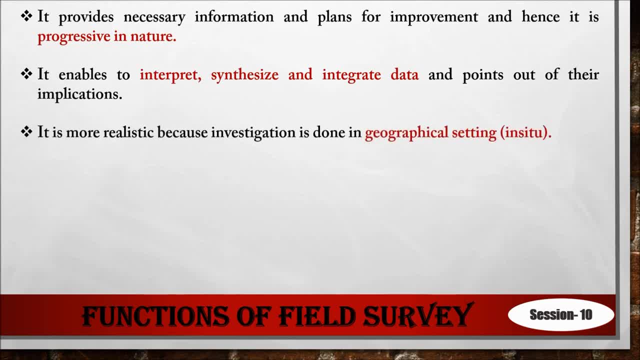 because investigation is done through geographical setting in situation, in situ. so what is happening in the context that we are studying? that's why study area is always a chapter in every report that we study in geography, right. so study area matters. geographical setting matters, right. it is the only method through which investigator or a researcher obtains opinion attitude. 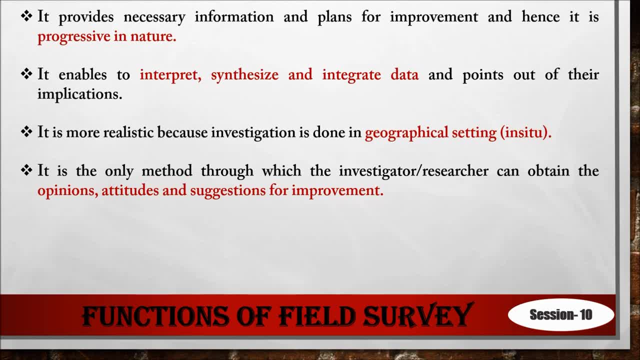 suggestions for improvement. this is what we aim to do, isn't it? so we study it and then we provide opinions, attitudes, suggestions for improvement in the ground situation. so it is useful in the developmental research process. so tools such as checklist method, questionnaires, schedules, everything you remember what we do is this is important for research development as well. finally, 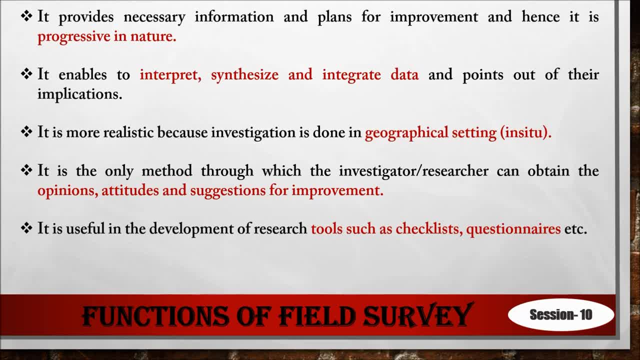 it may be- may not be- depends upon the quality of research. but larger picture is also to help to aid the agencies in decision making right. they can formulate strategies based on somebody's research of the ground in order to improve the situation on the ground if there is some problem happening. 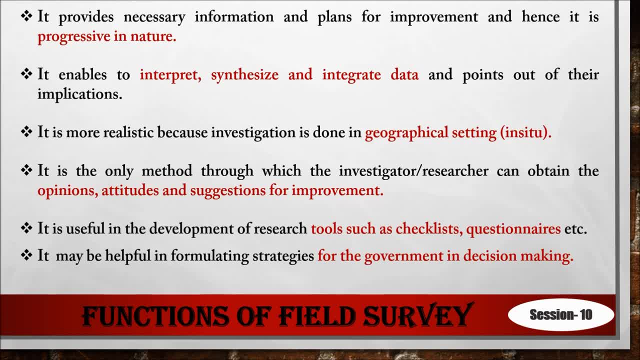 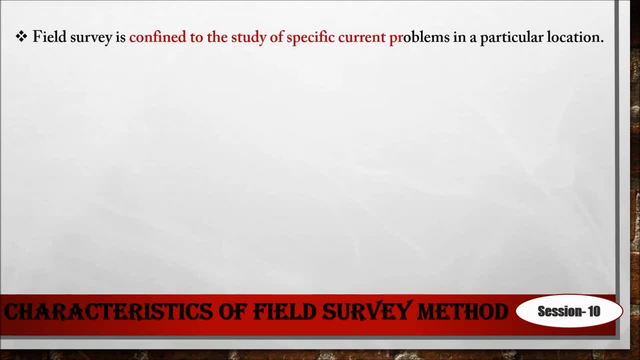 so these are the larger functions of a field server, right? so we understood the concept. then we understood the objectives, the functions. now let's look further at the characteristics of the field server method. so field survey is confined to the study of specific current problem. so the problem has to be specific and current, right it is: planned collection of data for predicting. 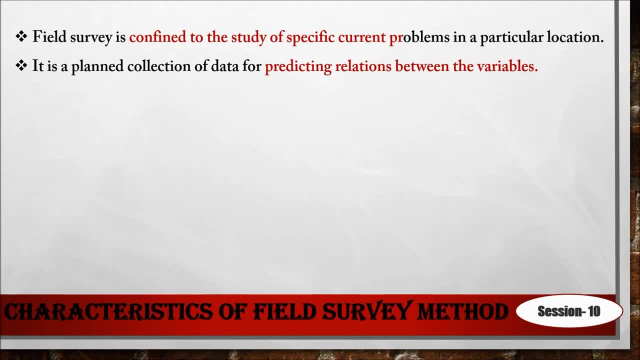 relations between the variables. obviously, we understand that there are various variables in our data sets and there is a planning in order to integrate, in order to interlink these relationships between the data. that's why static analysis comes to the picture, isn't it? then it is concerned with a larger, wide, 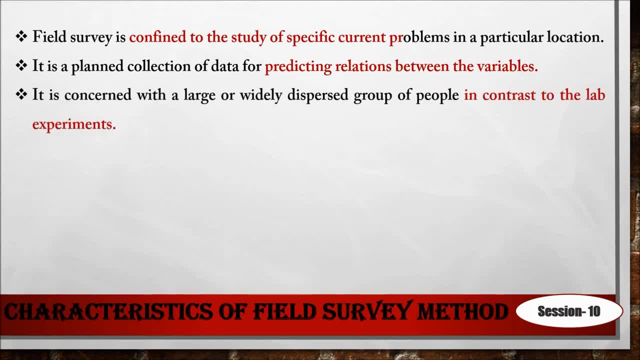 variety of group. obviously it's ground situation: a wide variety of people. so much of diversity there. so in contrast to lab experiments, in lab experiments it's very controlled, but diversity is more when we go to the ground situation. so under this method, observations, interviews, focus group discussions and 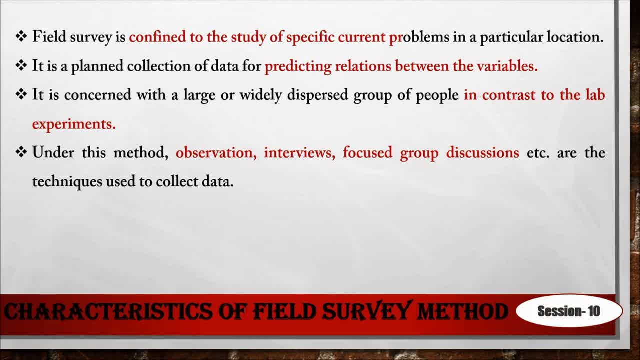 so many methods that we study are utilized to collect data right, these basic idea of observations, interviews, discussions, questionnaire, surveys, schedules. we are going to discuss that in detail in the next lecture, in details of the method of collection, their merits and demerits. so these are the important. 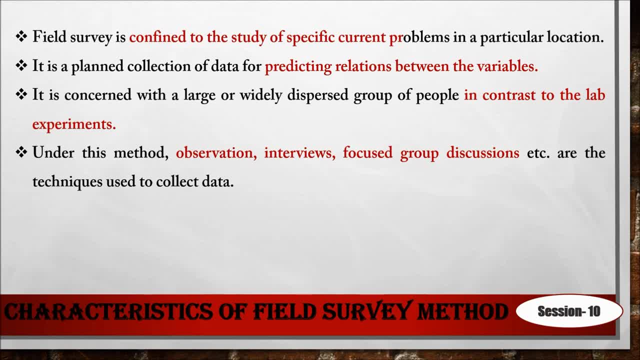 points. these are important characteristics we must understand right. the facts collected at one field, location may form the basis for social science research. so when we come from the ground, bring out certain information that can be the basis for other researches. so remember, you are, you have to be responsible when you are bringing out. 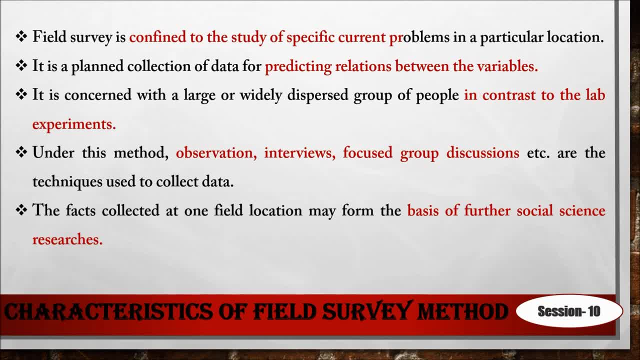 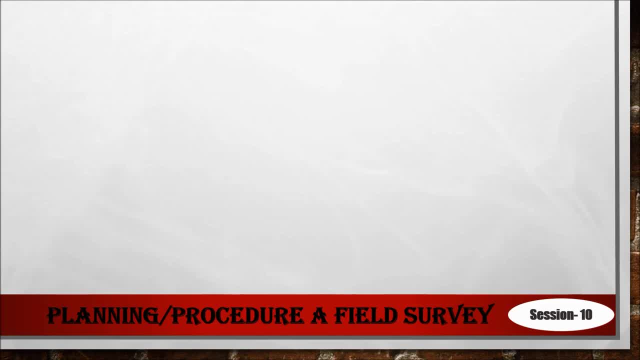 some inferences from the research on the ground. that's one of the characteristics. right now, let's look at the planning and procedure of a field survey. how do we plan? what is the procedure of planning of a field survey? so let's look at it. first important point is the selection of our research problem. okay, so we begin. 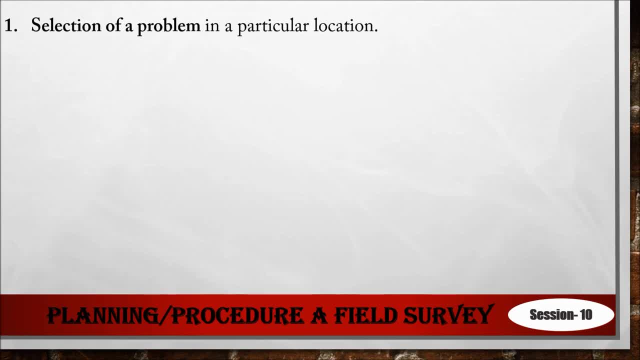 with a particular problem in a particular location. okay, so we begin with a particular problem in a particular location, and so suppose we look at the capital of India, that is, New Delhi. then we talk about problems. so problem is maybe air pollution, or we are talking about water. 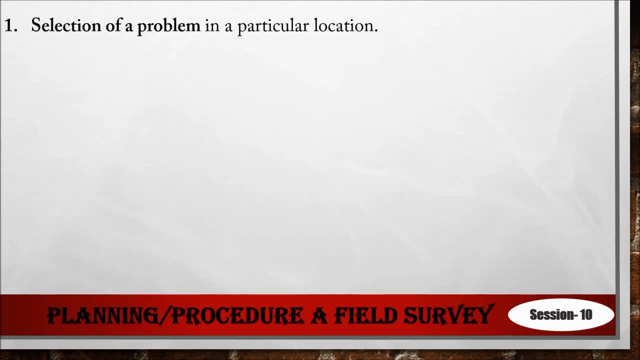 pollution suppose. so Yamuna side, if you take about. so the area is clear that Yamuna. now we have to be very specific: Yamuna, specifically in a particular location of the entire stretch of Yamuna, that is, in the Delhi NCR. so we need to be specific about that and exactness of the problem is important. so what kind of 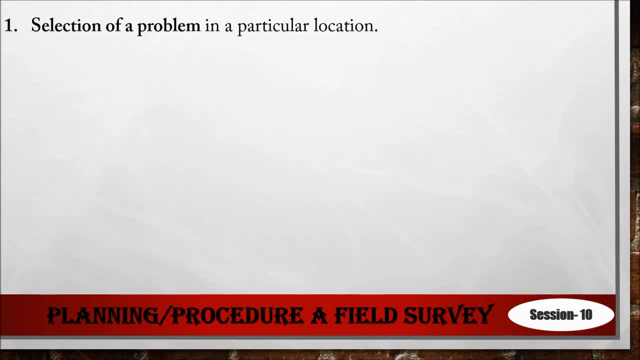 problem are we looking at right? so is it industrial pollution or is it water pollution or the severe pollution or maybe any other kinds of pollution that we study? and that is the example. so we need to specify our research problem and our such area location. then preliminary or pilot study. so preliminary study or 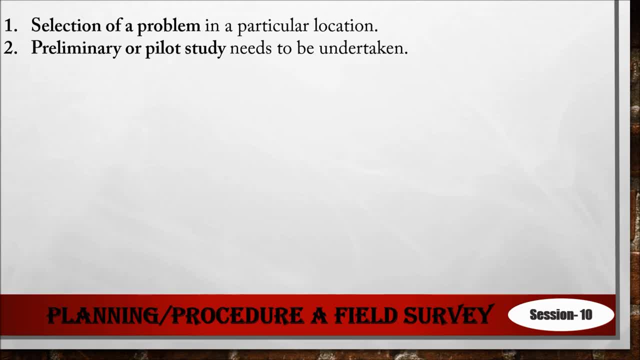 the pilot study is important to formulate hypothesis. we need to get a little hold of our situation, the problem, the idea of the area, isn't it? blindly we cannot step forward. so preliminary study is also important, but that also depends upon the time framework. if we don't have 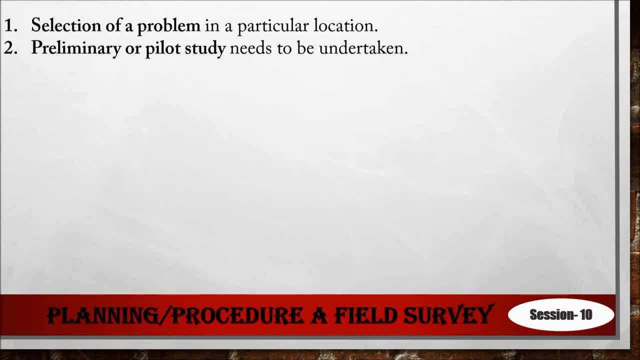 time to first do a preliminary survey. then we need to directly venture into the field. but preparation is important, so general and specific objectives have to be clearly framed and defined. in this situation, then it should be defined in a way that it is having adequate techniques of collection as well. so we 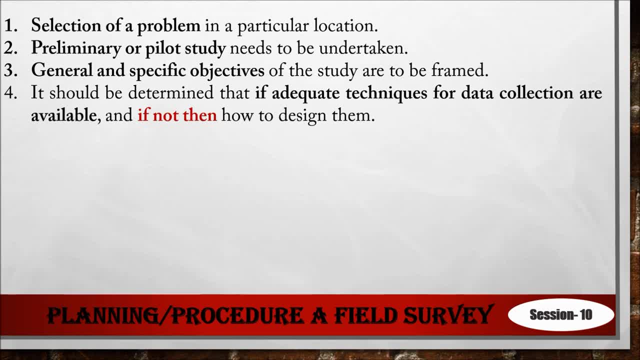 cannot randomly decide: okay, we'll go to the field and we'll collect this kind of data, but we need to understand that it has to have a design behind it. how are we going to do it? are we having adequate techniques for the collection? and if don't, then we need to design those techniques right. so that is very much. 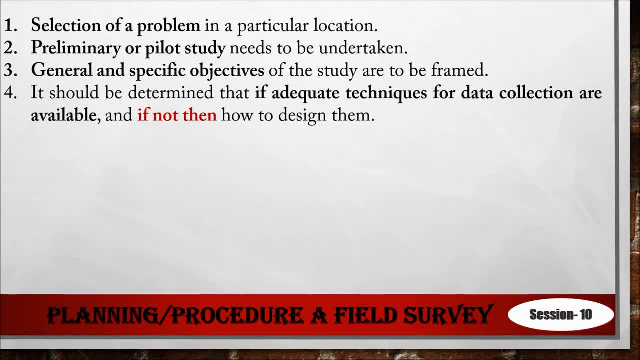 important. then we have population that should be clearly identified. now here comes that we have studied in the earlier sessions in sampling method that a sample should be very specific. we need to be very clear of the method of collection of data, so data collection design should be prepared as. 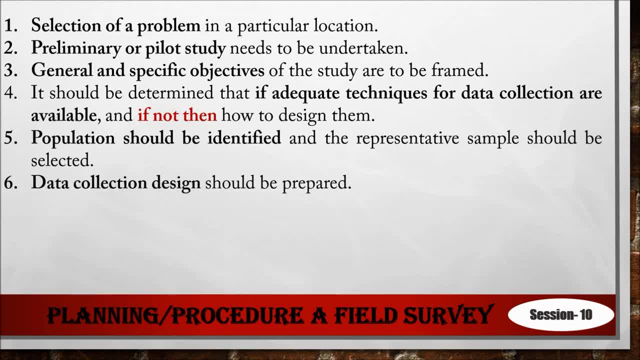 a handy tool, right? so data collection design is what we need to work out before going to be feel that's in the planning stage. that's the planning stage. the data should be collected through field survey methods. these methods, specific lecture. we are going to do that in the next session, in session 11. so 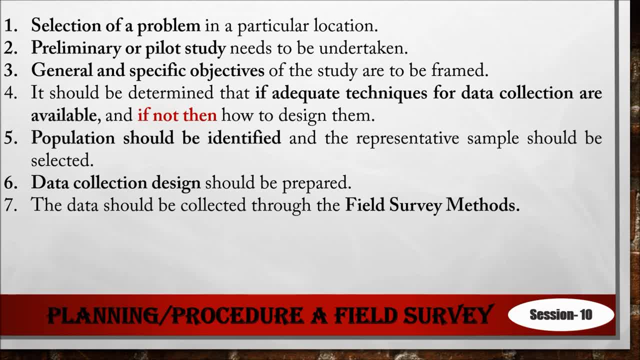 we'll be talking about there in details. then the data should be analyzed using appropriate analytical tools. now we are going to also focus on what are the tools of analysis in the upcoming sessions. so remember these are the important procedural part of planning a survey. the report is the last segment, so 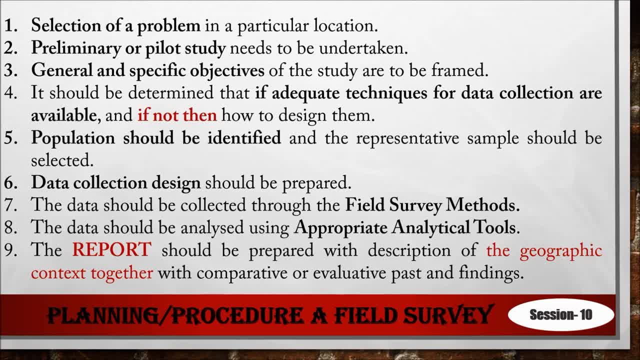 report should be prepared with a description of geographical context, together with comparative or evaluative understanding and findings comparisons. so it should be very clearly comprehensive in the context and it should have the inferences very clearly stated. so as of now we will be doing next sessions with field survey methods specifically with their merits and 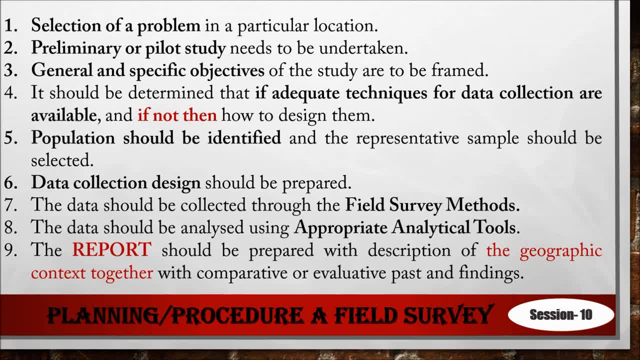 demerits. then we'll be talking about tools, will also be talking about the how to store data, the various applications that can be used in technology, and also then we'll go to the conventions of writing a report, how to design a report. so these are the basic ideas of planning of field survey. these nine points summary you. 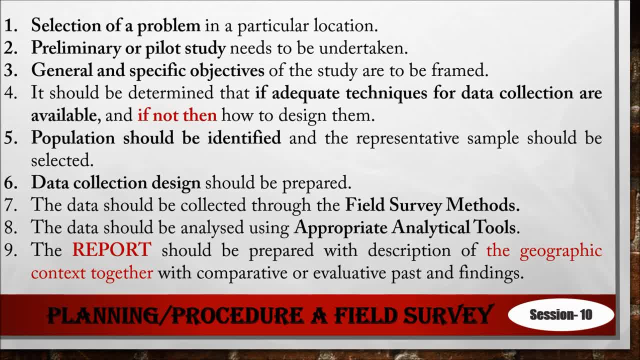 must remember that before a field survey we must understand to frame these nine points, to find answers for these nine points, if these are nine questions that we must have answers for to actually plan a good field survey all right now. so merits of a field survey can be: it's basically a close contact based 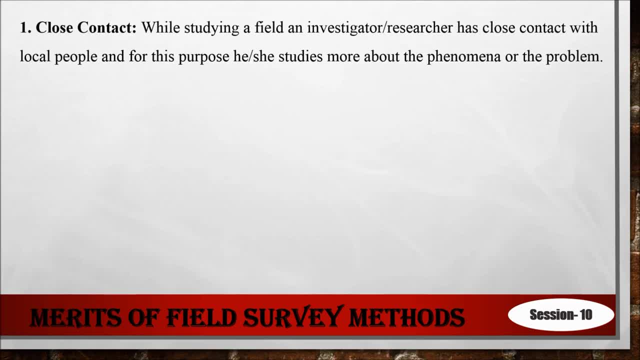 study, so that is very much important in the phenomena. a researcher or investigator has to have a close contact with the people. that is one point and that's why that can be a good study. greater objectivity- so field survey methods lead to greater objectivity- means objectively you can state a. 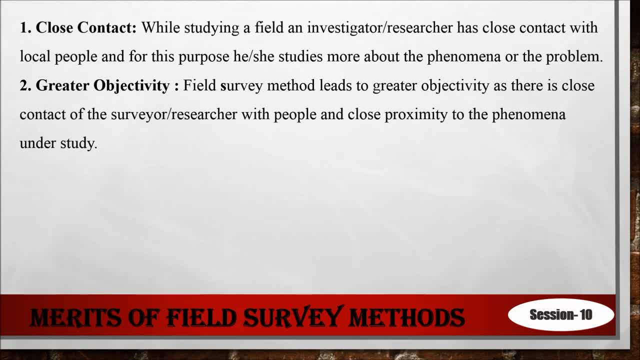 problem. you can say that, okay, this is happening, so we should be doing this kind of study. so close proximity with the phenomena under study. you can have a greater objectivity about the phenomenon. you can reduce ambiguity and subjectivity. right, this is a good merit of the field server method. then knowledge about a social situation: this is 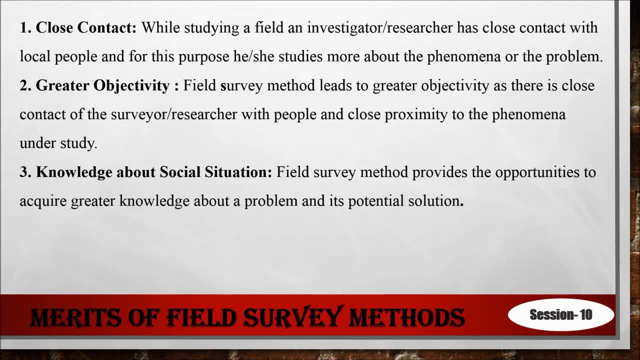 very much important in today's context: society, people. they are very much important and knowledge about the social situation in that particular context becomes one of the very much handy tool for a problem and its solution. right then, meticulous study of a problem because it's very specific, it brings out the meticulousness, importantly, because it is bringing out the cause. 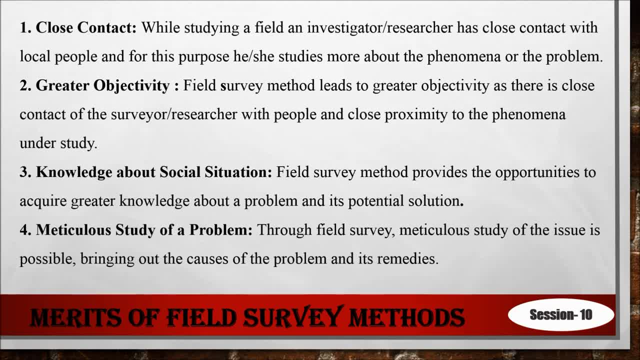 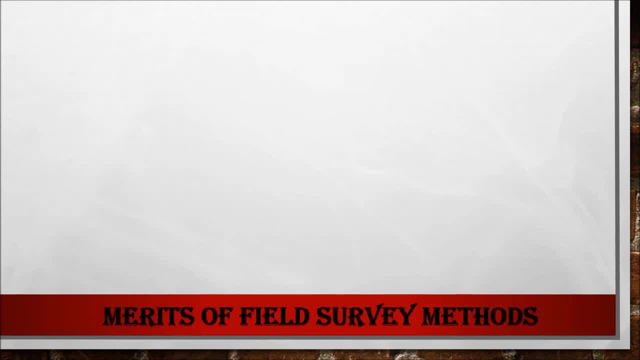 and effect relationships, the problems and its remedies we are talking about, isn't it so? that's why it becomes more important, then further. it's important for the administrator and policy makers, as we have already understood that these study would enhance the administration, the decision making of the policymakers and administrators. so in many countries, 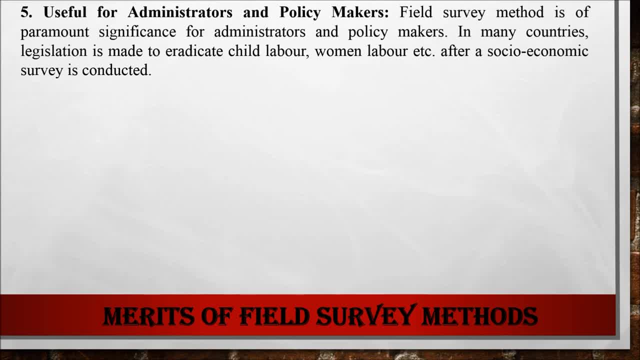 legislation is made to exactly child labor, women labor, etc. Socio-economic survey is conducted in that context. So many a times these surveys help us to formulate strategies as administrator, as decision makers, right, social change and development. Obviously, when we understand, socio-economic survey leads at finding, providing insights. 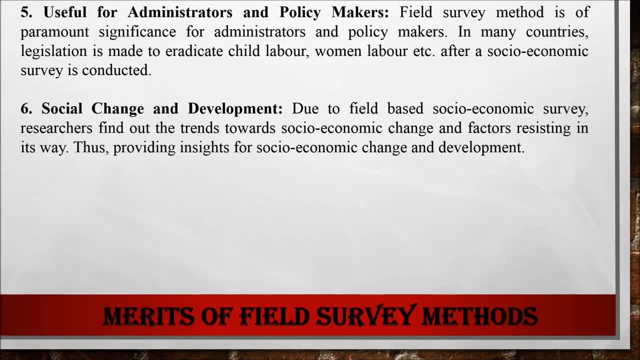 about the socio-economic change and development. So we are always defining and redefining, mapping and remapping the development course and we always tend to understand the socio-economic change right. So that's another positive point. Then more information and facts. So field survey is mainly the main source. 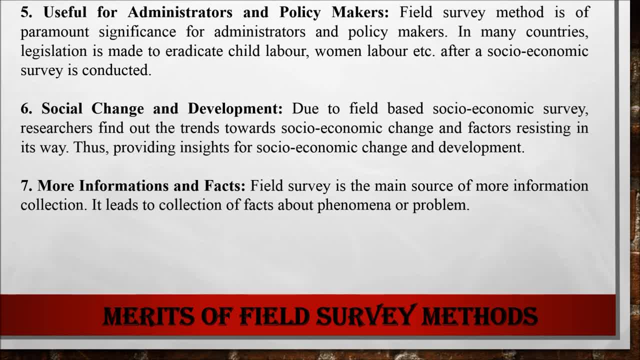 of the further information which is already not published, not there in the secondary data sources, isn't it? So it always gives us insights, more information and facts. okay, Then universal application, So it can be applied to similar jobs, geographical areas, entire world. if we understand that Geographical areas can, 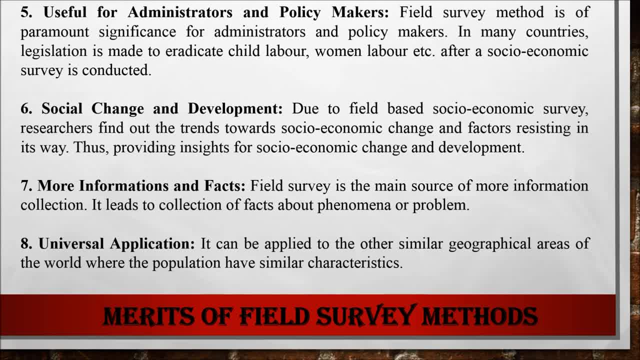 be similar. So if it is a similar area, so similar methods can be applied and population characteristics can be understood in a particular context. So if the context is same, then same kinds of methods can be used. So what can happen? There can be a universal application of field survey methods, isn't it So? if we 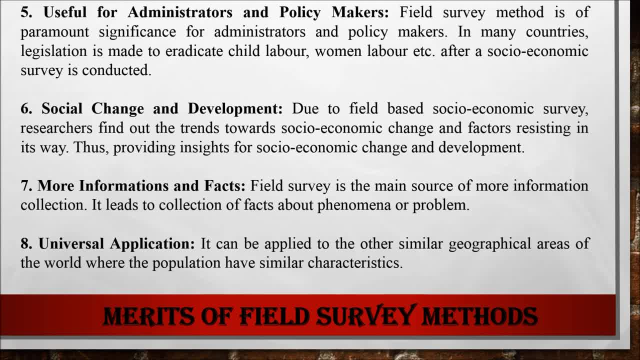 are doing a questionnaire survey in one part where there is a particular site situation association. same site situation association can have the same kinds of questionnaire survey universally. So this is very much important to understand that field survey methods are also of a universal nature, especially in social science and policy research. 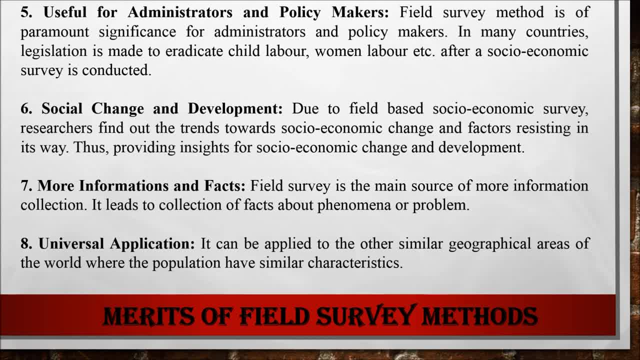 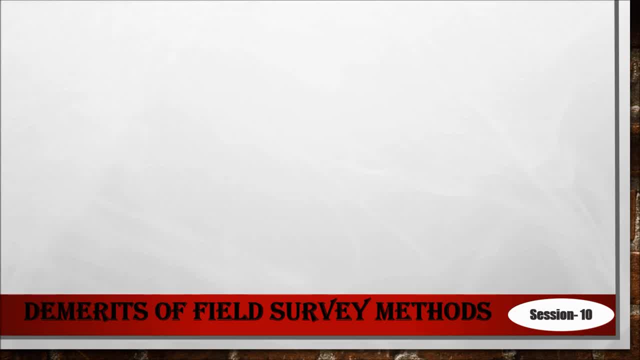 alright, Now let's look at certain demerits as well. We must understand that there must be some demerits. We must take care of these demerits while doing a field survey. So one is specific training. So it is important that if we don't have 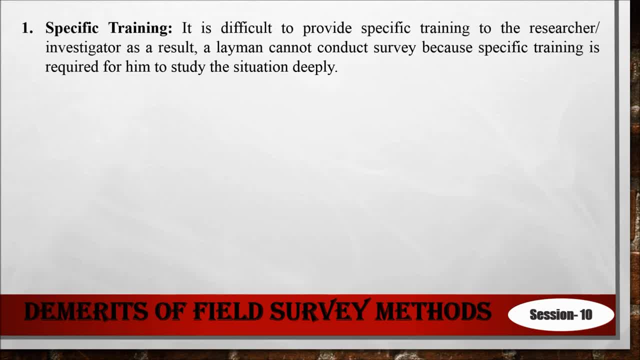 specific training. we must take care of these demerits while doing a field survey. So one is specific training. So it is important that if we don't have specific training, we We must understand that a layman cannot conduct a survey because it has a specific nuance. 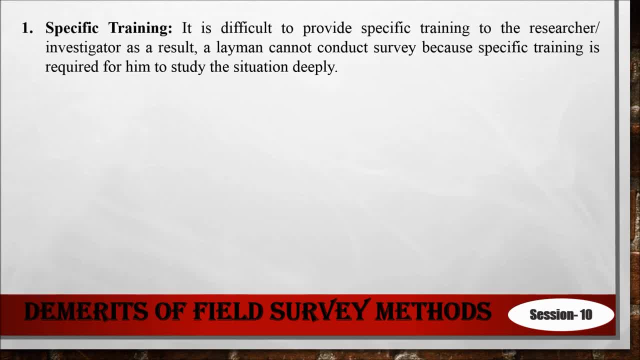 of study involved in it. So there will be difficulty if you are not trained for the field survey. So we must train ourselves for a little survey, by preliminary surveys, by reading, by doing certain exercises so that we can understand how to conduct a survey. 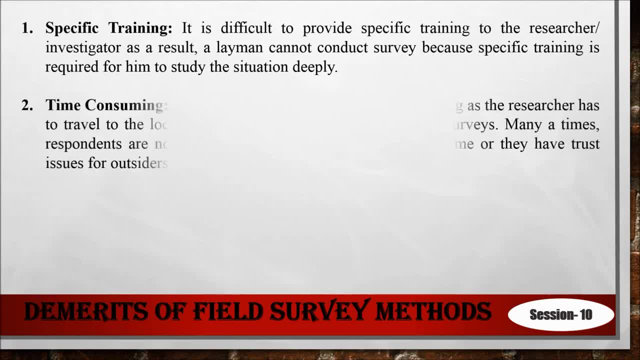 It is time consuming. It's very much important that if we don't have time to go to the field, then many a times we cannot come with good surveys in short time. Many times what happens if you go to the field? people are not ready to respond. 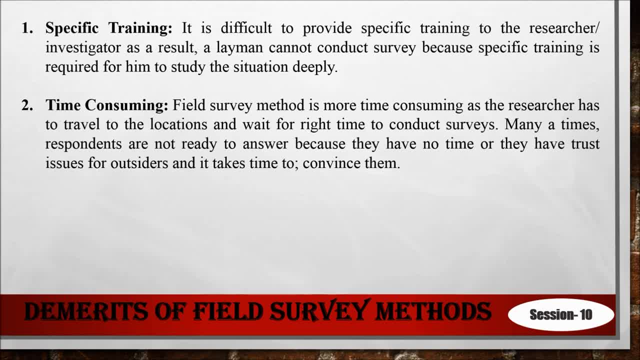 So you have to go again and again. So time consuming factor is a demerit. Again. cost money, grant finance. it's becoming one of the most important point in today's world right. So the higher expenditure of research investigator becomes many times a limiting factor. 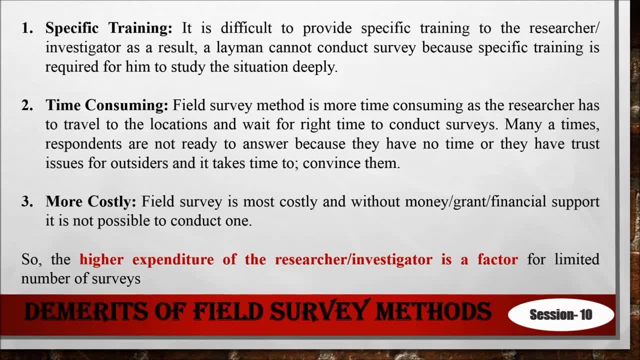 Who is sponsoring you? Who is doing the financial part right? It has a cost involved If you go to the field, So that's also very much important to understand for a researcher. before going to the field, In the planning stage these demerits have to be taken care right. 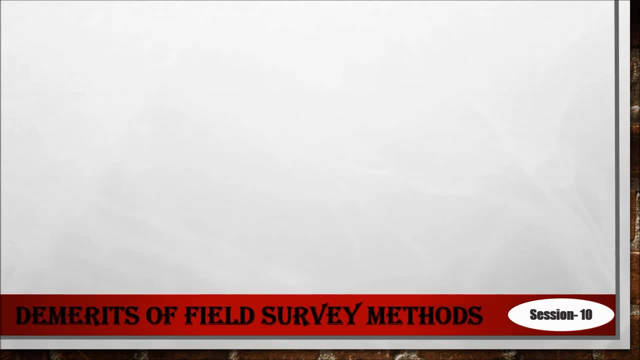 We must understand that there can be a sampling error. We already did that in the previous sessions, That sampling errors are very much to be avoided because we must understand that in what context, what kind of sample will be used and what is its demerit. 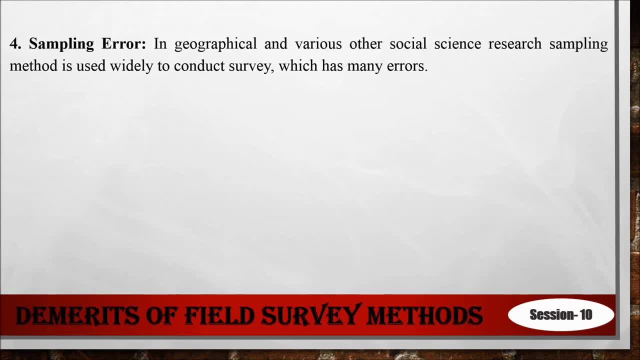 So error has to be minimized in order to good results, right, So for good results, errors have to be less. No application to historical problems: Many times what happens, these field survey methods don't have anything to do with any historical solution of any problem, because it's very much based on the current situation. 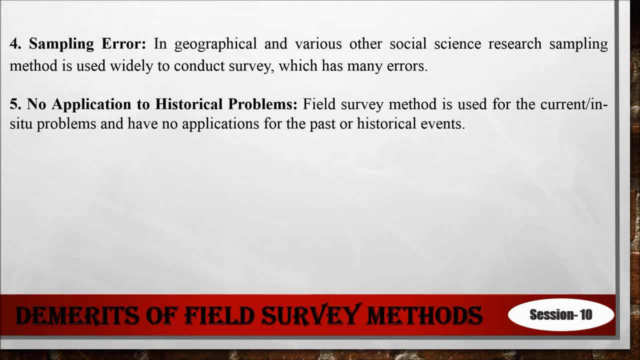 in the present context of the study. So many times any historical problem cannot be addressed. That can be a limitation. Again, data uniformity may be problem because there is no uniformity in data many times in our field survey methods. So it is because of the diversity of the respondents and also many times discrepancy of the respondents. 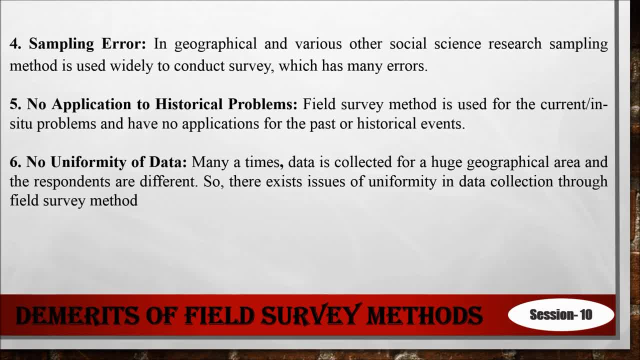 idea of what we are going to ask them. So what happens? We are asking them a particular context, suppose climate change. So we are asking them a particular question, a particular type of question in climate change, and they don't understand climate change. 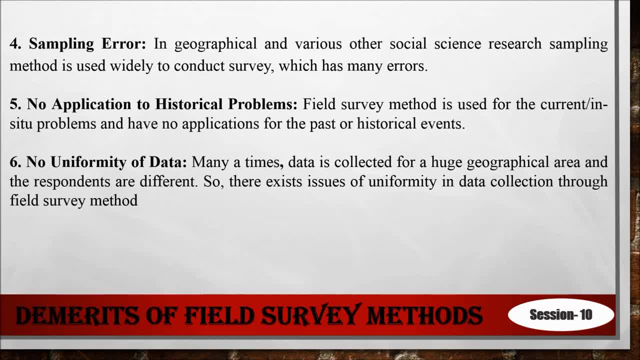 They would answer you in their ways of understanding. So what happens? There can be a discrepancy, So data uniformity may vary. Somebody survey in a climate change can be different than your survey in the climate change. So this is what happens. because of this non-uniformity of data, there can be a certain limitation. 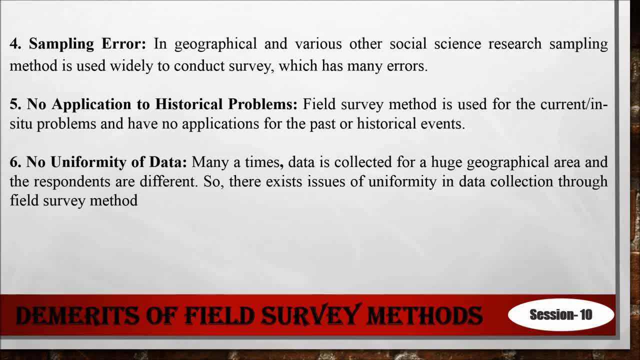 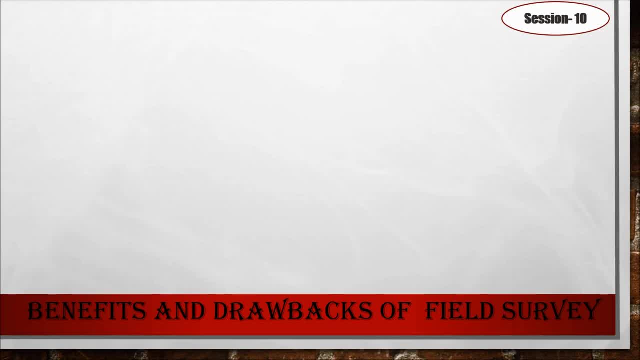 to the study. Now we will understand this entire summary of the benefits and drawbacks through this flow diagram. So what we are talking is the benefits on one hand and drawbacks on one hand. So benefits says it is current, it is generalizable, it's versatile, and drawbacks are cost effectiveness. 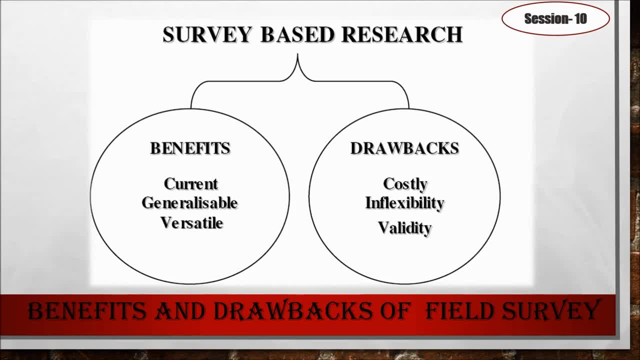 is a problem- inflexibility right, So it has to be a particular context and flexibility is sometimes important. It's an issue and validity. many a times it's an issue because of the certain issues that we already talked in the demerit section. 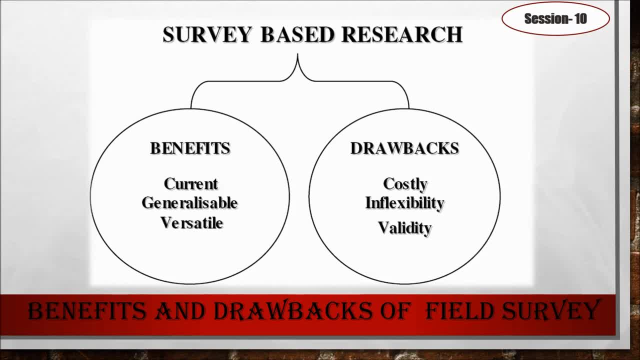 So if we understand the benefits and drawbacks both, then we are better versed, we are better equipped to carry on our field survey. So today's session was basically meant to understand that before going to the field we must understand the conceptual part, the merits and demerits part, the benefits and 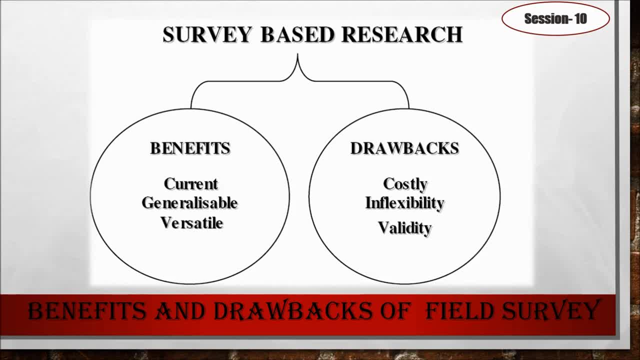 drawbacks, part And point wise analysis of every section of the structure, of the function, of the planning, isn't it, before going to the methods, actually, that we're going to do in the next session? So please continue to learn a lot, and the next session we are going to come with the